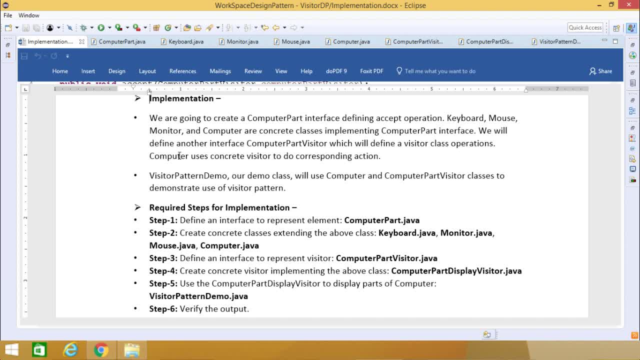 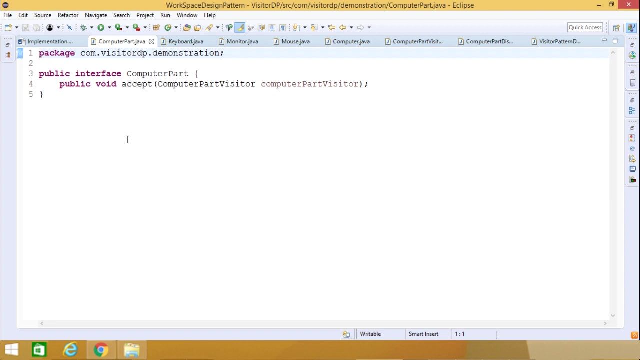 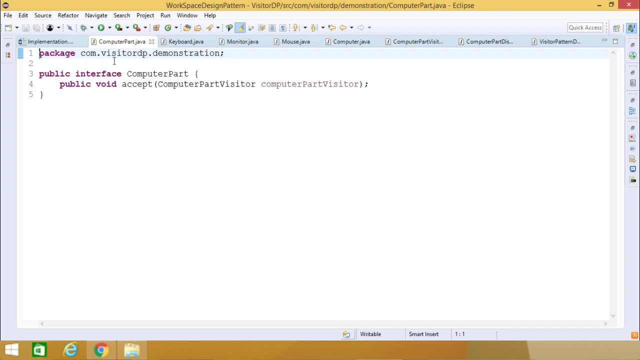 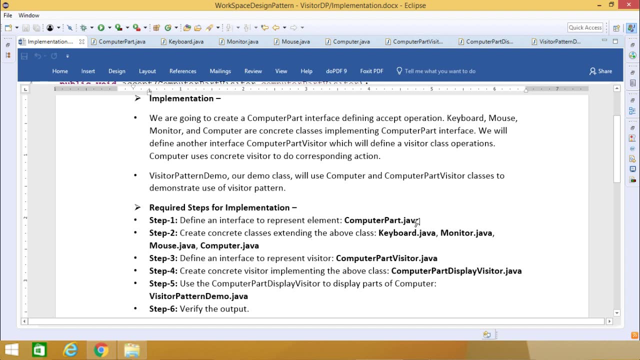 unimplemented method: accept. you can see the code here. now, going for the step number two, create concrete classes extending the above class, that is, the computer partjava, and the extended concrete classes will be our keyboardjava, monitorjava, mousejava and computerjava. so going for the 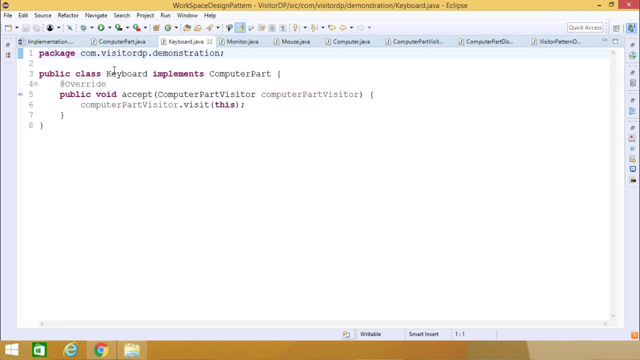 keyboardjava. so keyboardjava, that means the class keyboard implements computer part, this respective interface, so accept method is to be defined here. so where we are having computer part visitor object will be the input parameter. so computer partvisitorvisit. this that means the object defined under this keyboard. that will be the input argument to this visit method. 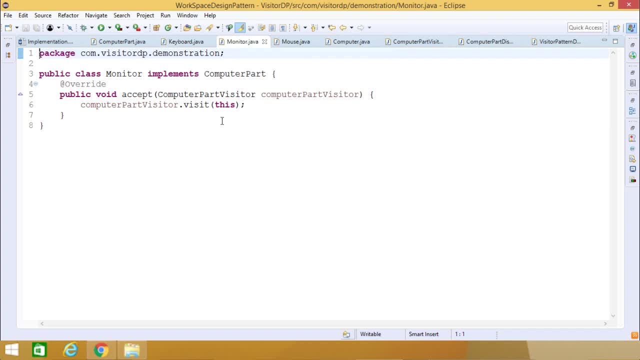 so now we are going for this monitor, we are writing the same, and here also we are passing this monitor class object as this input argument to this visit method. similarly, for mouse we are doing the same. and computer. now, in case of computer, you know that computer will be consisting of multiple parts. so here we have defined one array of computer part. 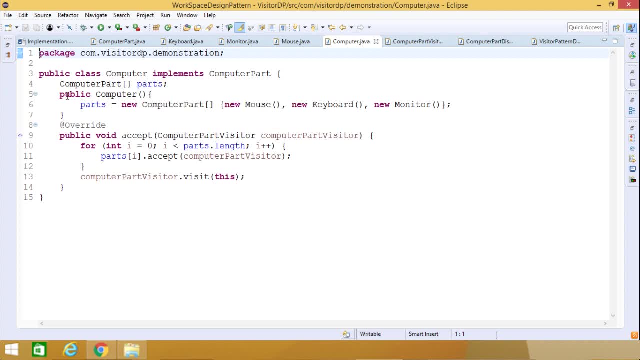 so name of the array will be parts here. so public computer, that is a constructor we are having. so parts is equal to new computer part. so what we are keeping here: one mouse class object, one keyboard class object, one monitor class object, and comprising them we are making this computer. 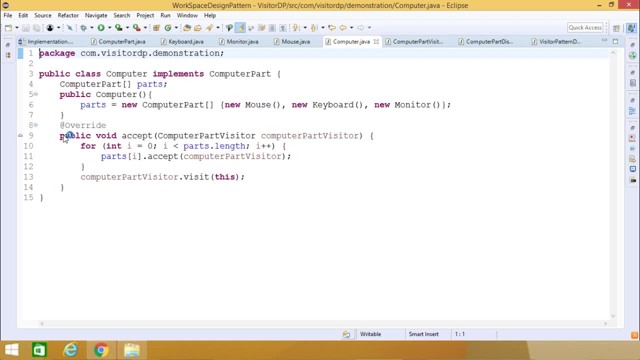 part array. there is a parts here. so now public void: accept: computer part visitor. so computer part visitor, because you know here also it is implementing this computer part interface. so as a result of that, this accept method must be defined there you. so that's why it is our accept method. so here we are going for: for i, int. i is equal to zero, i less. 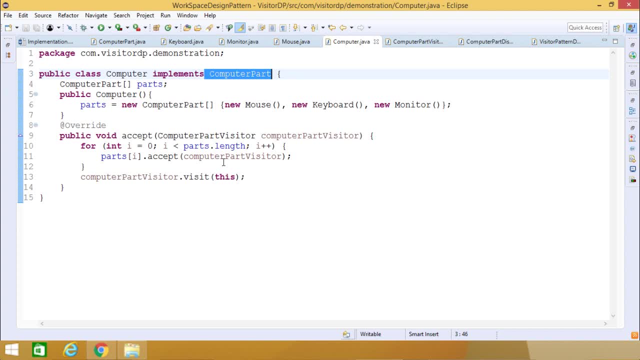 than parts dot length. we know that parts dot length will be the value three. so i will be ranging from zero to two. in that case i plus plus parts dot. i dot accept computer part visitor and then we are having this computer part visitor dot visit this. so whatever the object we are finding, so that 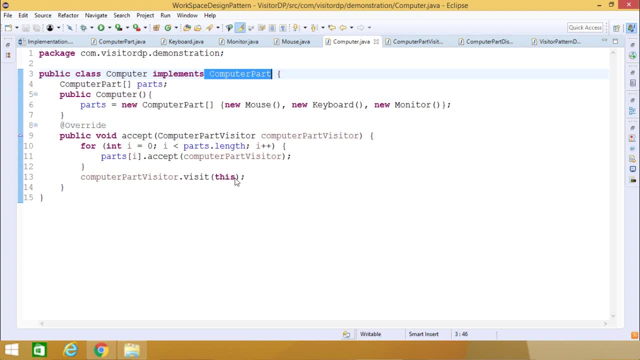 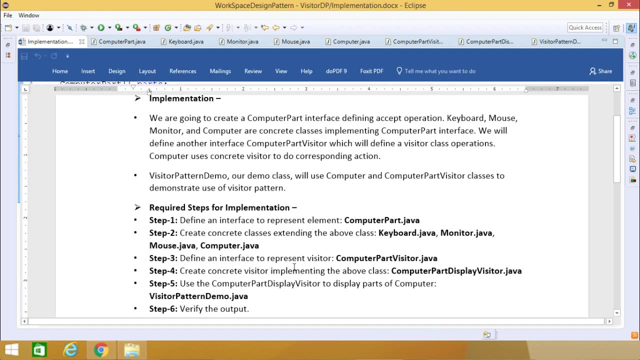 means the respective computer object will be passing as input argument to this visit method. so in this way we have done, we have written, now, going for the step number three, define an interface to represent visitor computer part visitor dot java. so in the step number three we are going to define one interface and that is the that will 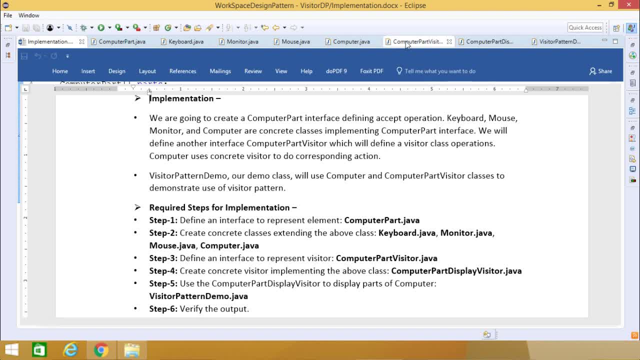 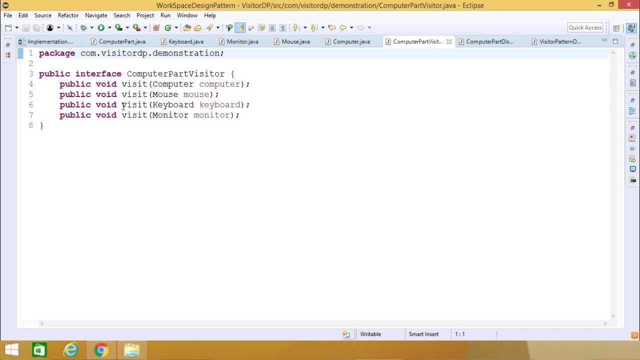 represent the visitor and that is a computer part visitor. so now we are having this computer part visitor. so here you see, in case of computer part visitor, it is having three methods. we're having, you you see, the same method but with the different prototypes we are having. so we are using the 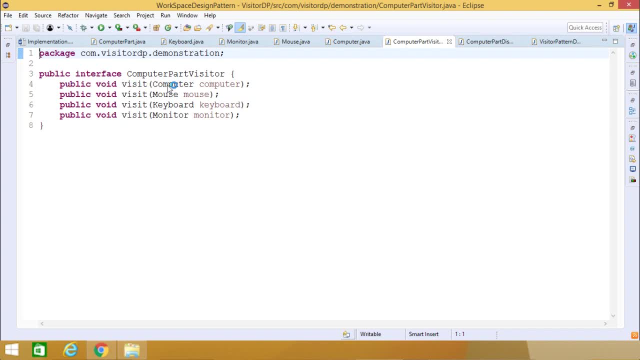 property polymorphism here. so public void visit computer object. public void visit mouse class object. public void visit keyboard class object and public void visit monitor class object. here you see, here we are passing this visit is taking the keyboard class object. that means this very method is getting executed in that case, but the here the method bodies we have been written. 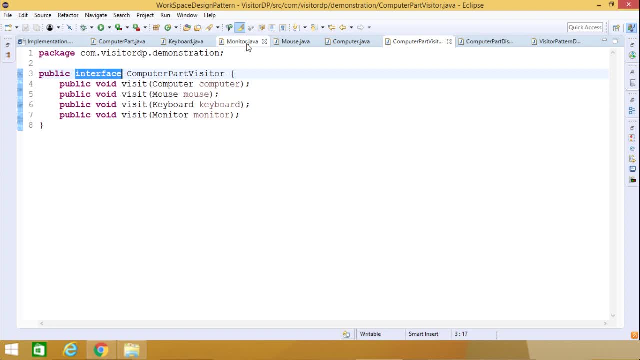 because it is nothing but a interface, nothing but one interface. so now, in case of monitorjava, we are passing this monitor class object as input document. so in that case you know that this particular method will get invoked. so i require one implementation class of this computer part. 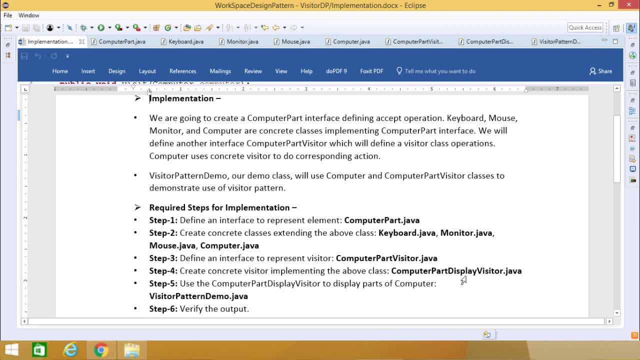 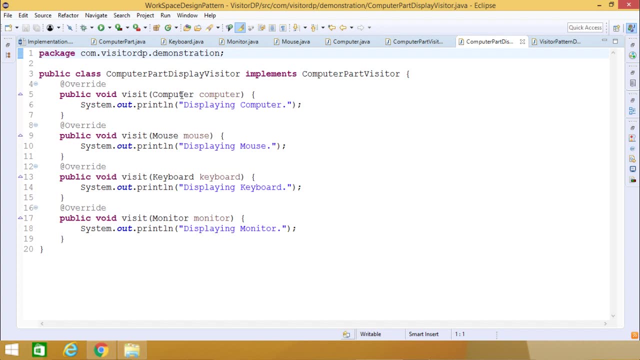 visitor. so now we are going for this, this one, that is a create concrete visitor implementer, implementing the above class, that is a computer part display visitorjava. so now let us go for computer part display visitorjava. so here this computer object is there, mouse object is there. 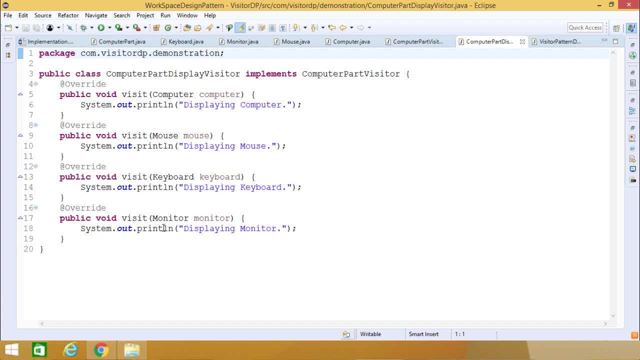 keyboard object is there? monitor object is there, passing as input argument to the visit function, and here we are using the property. we are implementing the property polymorphism here. so here we are having systemoutprintln, a very simple messages are getting printed and meaningful and logical messages are getting printed, depending upon the respective input argument. whatever has 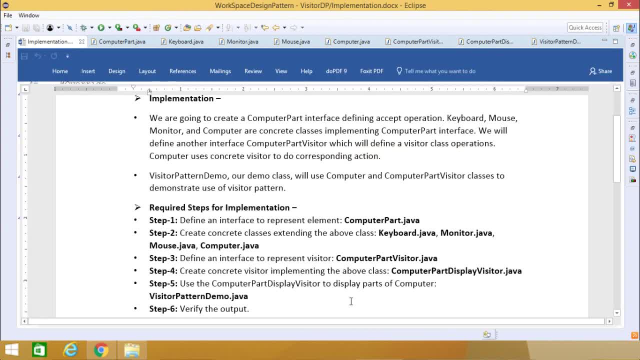 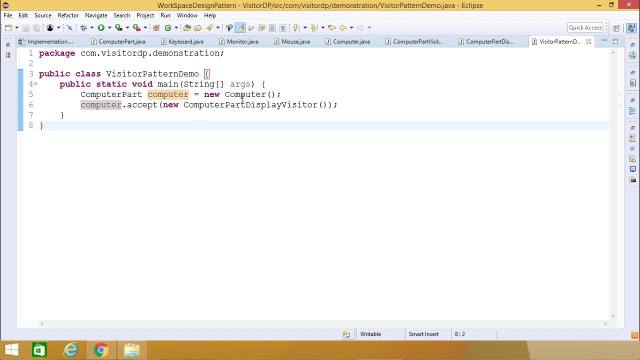 been passed to the visit. so we are going for the step number five. use a computer part display visitor to display parts of computer. so visitor pattern demojava. now going for the visitor pattern demojava. so here we are having this computer part. object is equal to new computer. and then 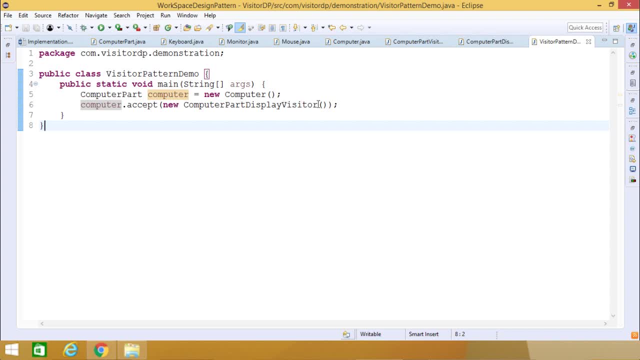 computer dot accept new computer part display visitor. you know that computer part dot display i use the computer part to display the new computer. the display visitor. you know that computer tab and display visitors is the new computer that we need to display everything that will come into the. allora, right now, that computer package aligned with the yaoh, the nav of our DJM and with a τα stream ayudar cave, is what we java네요, the java of our js share of the intuitive inside freedom is a new computer is equal to needs three components. it is a new component, so with our java we need to go for. 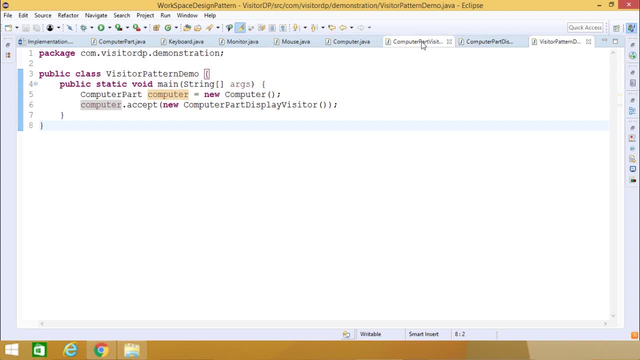 that computer part display visitor is nothing but the implemented class of this interface. implemented class of this interface. so what will happen in case of we are having this computer dot accept, we are passing this computer part display visitor because you know that in case of computer part this accept method was there undefined and here it's supposed to take computer part visitor. 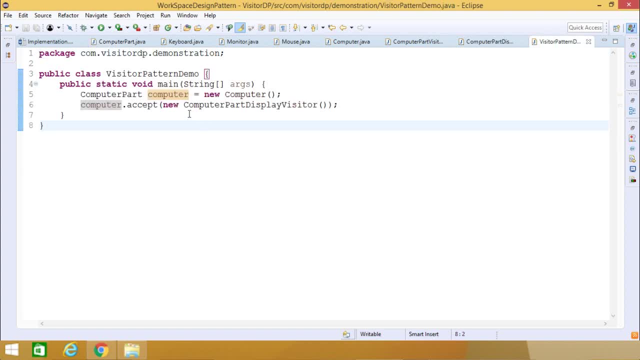 interface object. but here we are passing this computer part display visitor object as input argument, because computer part display visitor is nothing but one implementing class. of the implementing class of the computer part visitor, there is the interface. so that's why we can pass this one as well. so now let us go for. so computer part is equal to computer, is equal to new computer. 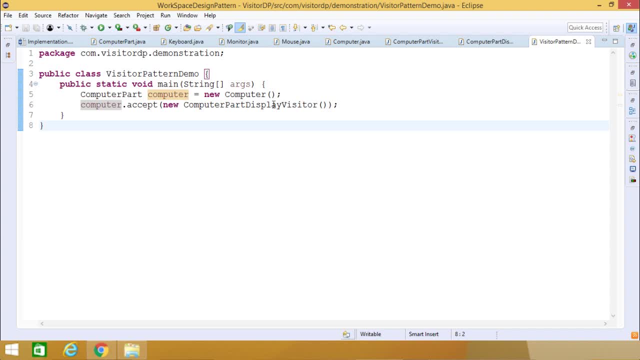 and then, from this computer dot, accept new computer part display visitor. now, going for this execution of the code, we are finding that display mouse, displaying mouse, displaying keyboard, displaying displacement, also displaying mouse monitor and displaying computer, so all these four messages are getting printed and that this message 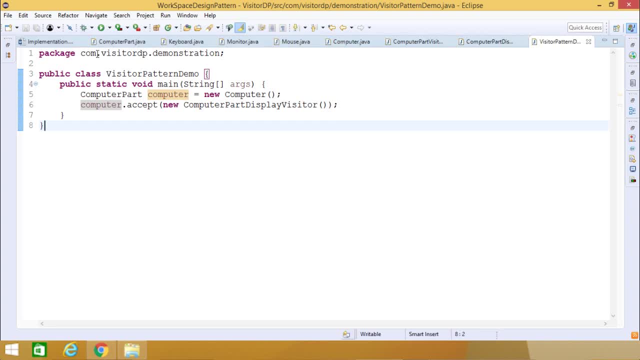 is printing is very much logical. and now let me repeat my explanation once again. so now you are finding that here we are having this computer part dot java, so it is having. it is one interface having one unimplemented method accept taking this computer part visitor interface object as input document keyboard is the implemented class of this. 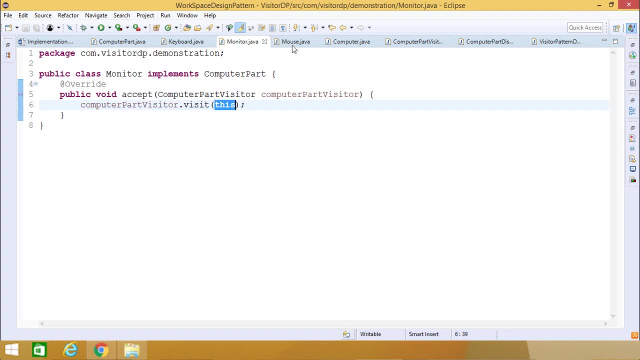 computer part. monitor is that one implemented class of this computer part. and mouse is also one concrete class implementing this computer part. and computer is also one concrete class implementing this computer part. and now we are having this computer part visitor. we have explained that one. we are having three, four methods are there? all of them are. 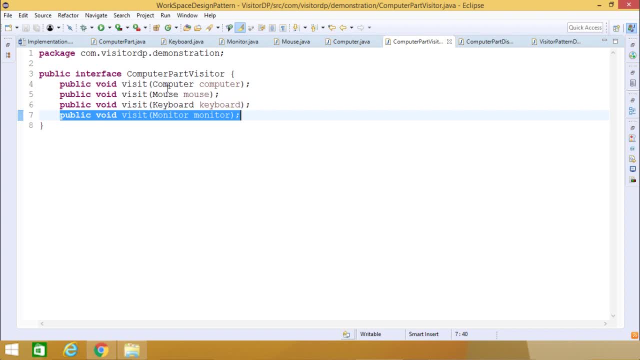 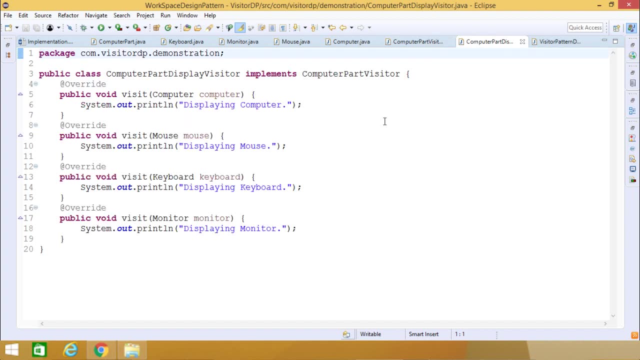 having the name visit, having this void as output argument. but their input arguments are differing and but that is one interface. there is a computer part display visitor. it is implementing this respective interface here and this: these are the respective functions the respective bodies have got written and there is a final one that is a. there is our, there is a visitor pattern demo. so 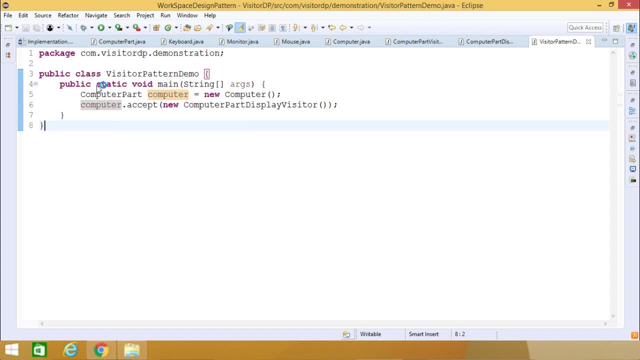 this is the class which is the last class and in this particular case we are having this main function where we are defining one computer part object and then computer dot accept new computer part display visitor. so respective object will be passed of this implemented method that is a computer part. 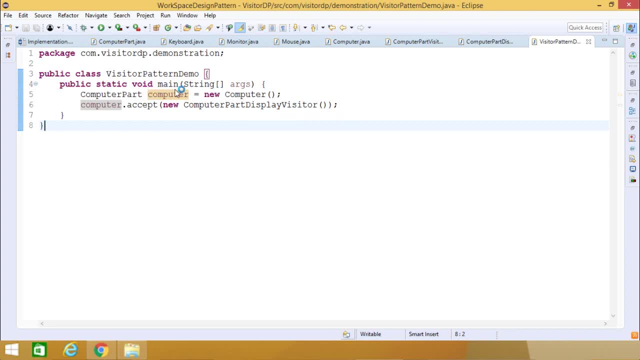 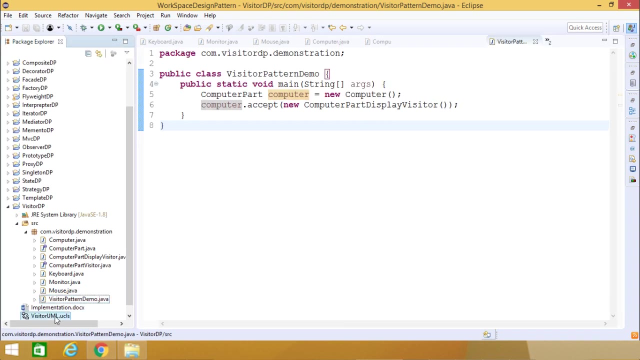 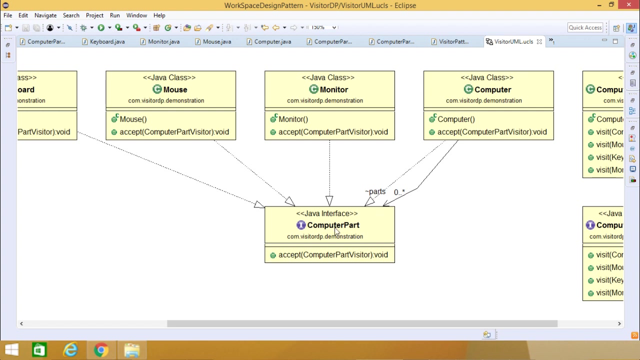 display visitor. so in this way my code is getting executed. i have shown you the output. i've shown you the output. now we shall go for the class diagram. so so this is our respective class diagram. you can find that this is the interface computer part, and these are the concrete implementing classes. there is a mouse, monitor and computer web. 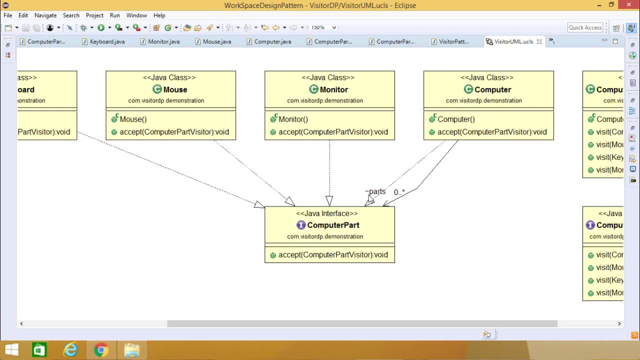 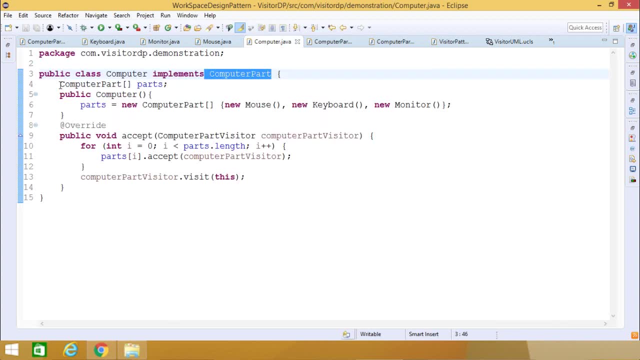 explain that one in case of computer. we are having this. there is a parse is there. so there is one parse. you can go for this computer. now you can see that we are having this parse which is computer part, this type of array. so it will be containing computer part objects in this particular array. so now we are having 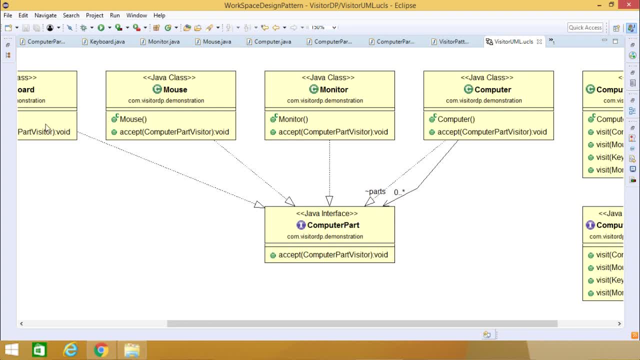 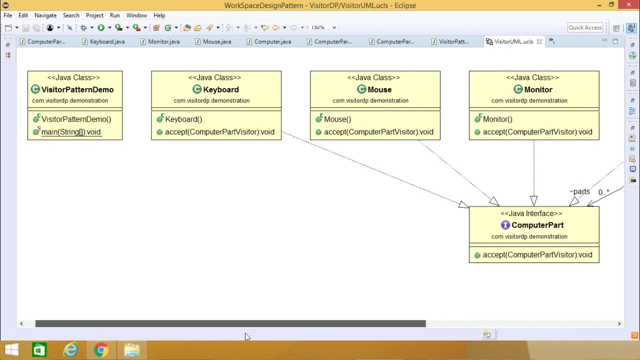 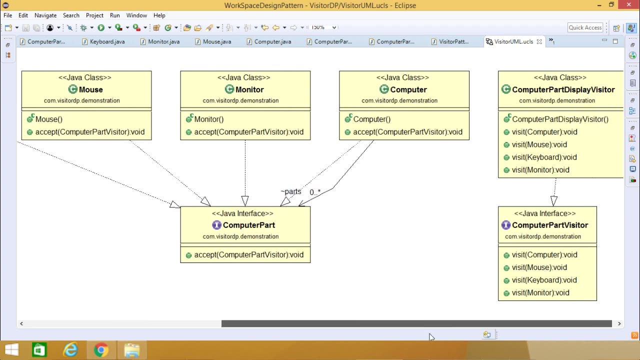 this is a parse- is there and we are having the. another implementation of this computer part is a keyboard. so keyboard, mouse, monitor and computer are the implementing classes. so this is a visitor pattern demo containing the static main function. and here we are having this computer part. visitor one: